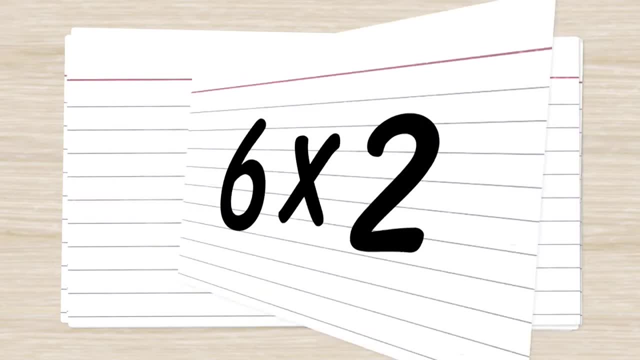 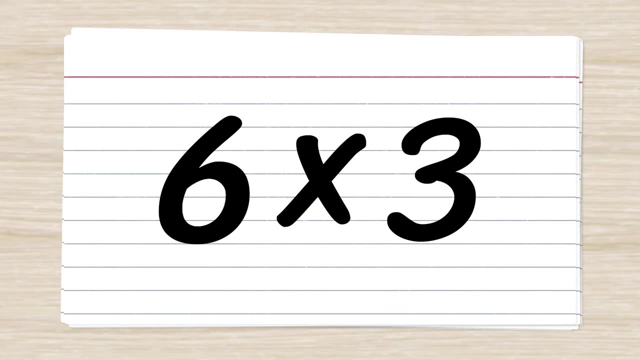 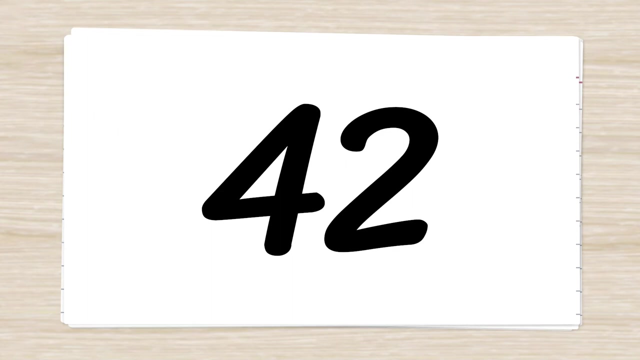 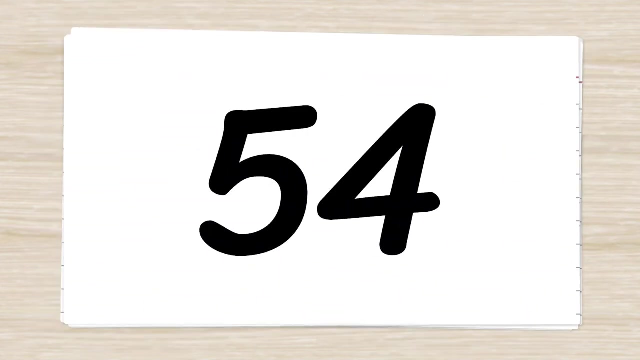 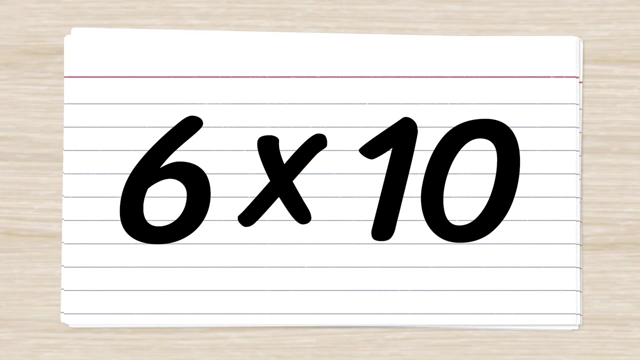 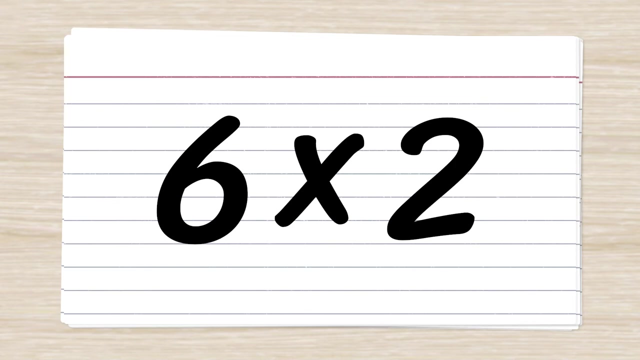 Twelve Six times three. Eighteen Six times four. Twenty-four Six times five. Thirty Six times six. Thirty-six Six times seven. Forty-two Six times eight. Forty-eight Six times nine. Fifty-two, Fifty-four Six times ten. Sixty Six times two. Twelve Six times nine, Fifty-four, Six. 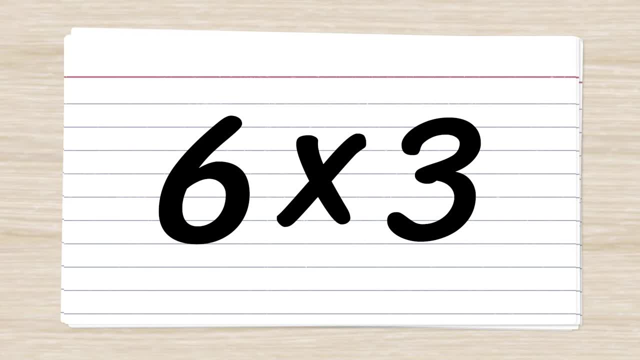 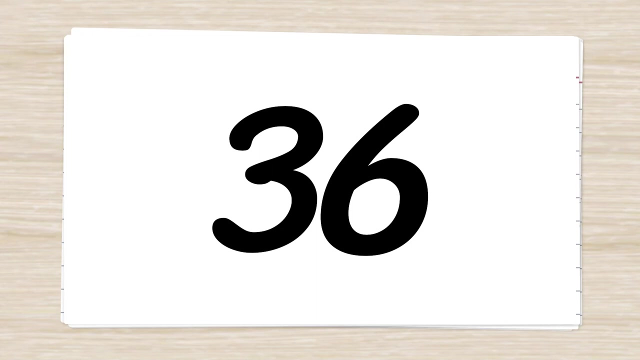 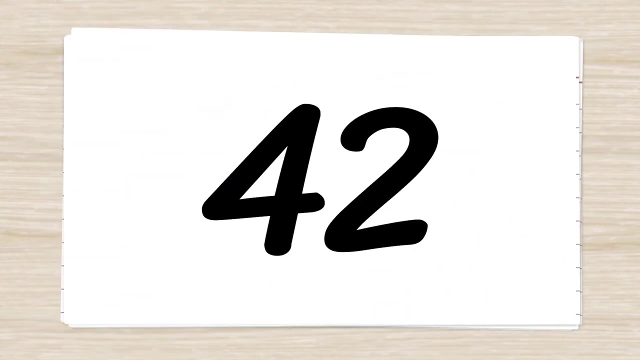 times three. Eighteen.06. Eighteen, Six times four. Twenty-four, Six times one. Six, Six times nine. Fifty-four, Six times six: 36, 6 x 7, 42, 6 x 8, 48, 6 x 10.